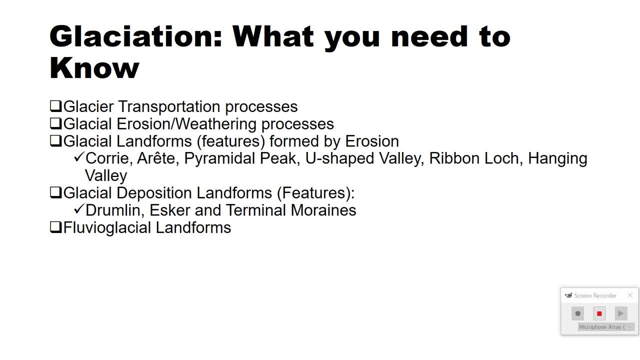 we're going to look at that form by erosion. We're looking at a cori, arret and pyramidal peak. They can be combined together. If you know how a cori is formed, you need a couple of extra sentences to form an arret or a pyramidal peak. So learn a cori very. 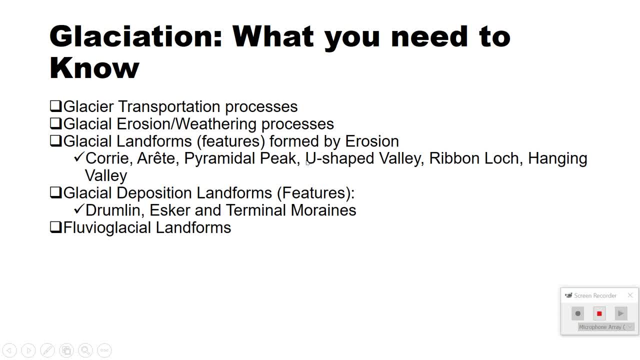 well. The same goes for a U-shaped valley. If you understand how a U-shaped valley works when you're giving an answer for a ribbon lock or having a hanging valley, you will use this answer to help create these ones. So these are two core features you need to know extremely well. 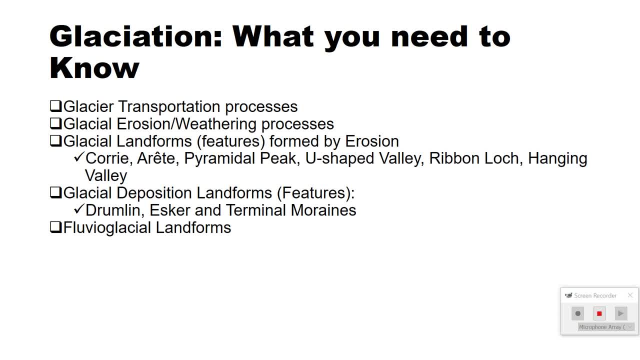 the cori and U-shaped valley Glacial deposition landforms that the next section we'll look at. we're only going to look at three of these. Two of them, a drumlin and an escar, are formed by- sorry. two of them- a terminal moraine and a drumlin, are formed by the glacier itself. 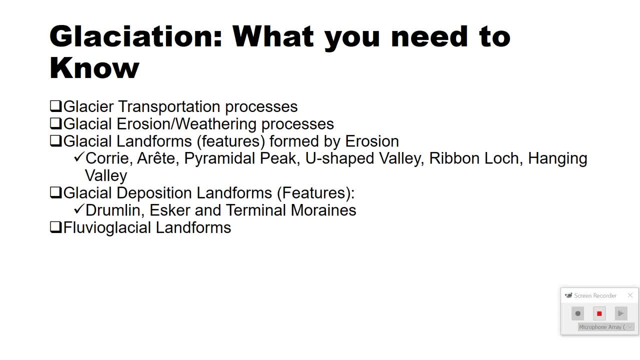 And then the escar is formed by water underneath the glacier or within the glacier, And so the escar is known as a fluvial glacial deposit- And we'll look at that later on- And that's a fluvial glacial landform which is listed underneath. 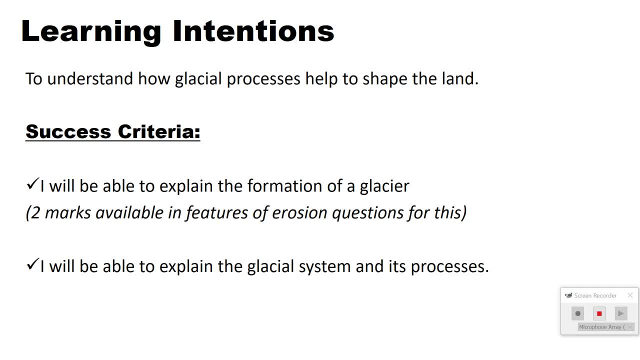 Moving on. So today's lesson is about glacier system. We just want to understand how glacier processes help to shape the land and learn a little bit about what a glacier is and how it works. You should be able to form talk about how a glacier is made or formed. Two marks are: 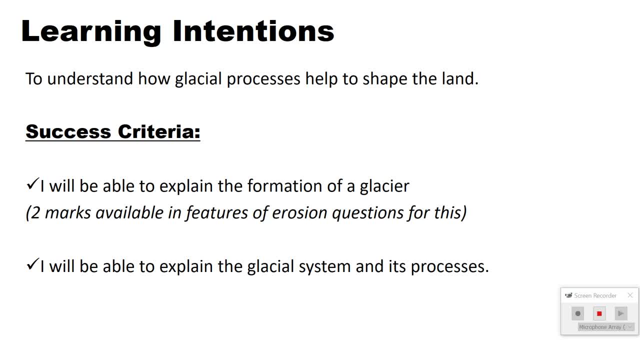 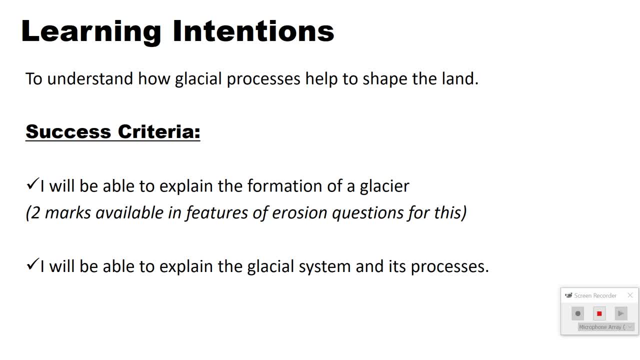 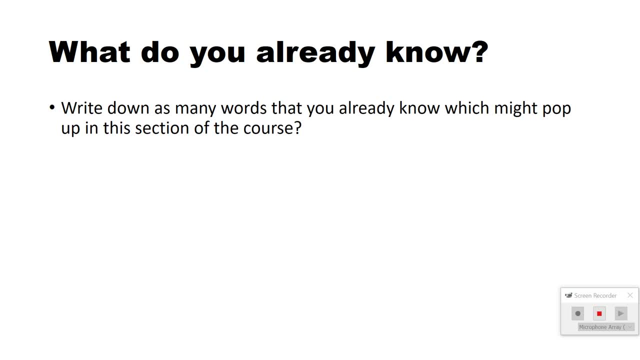 really easy marks to pick up. I'll be able to explain the glacial system and its processes, So that's sort of key learning for today. you should be able to do. What do you already know? Just now, you can pause the video and just give yourself. write down in your notes as many words as you. 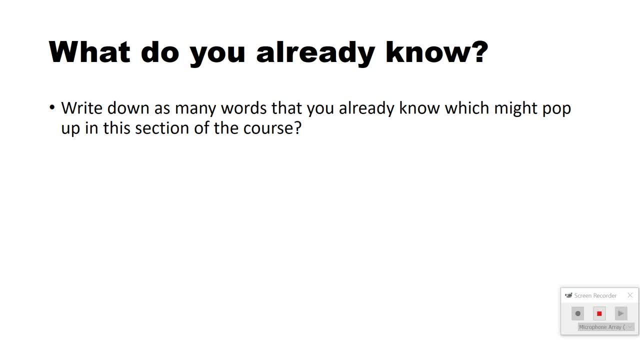 already know which might pop up to this section of the course, And you can unfreeze when you're ready and carry on with the video. Glacial terms: go in, learn these. You'll come across them throughout the different lessons And I may well give you a glossary to go and have a look at. 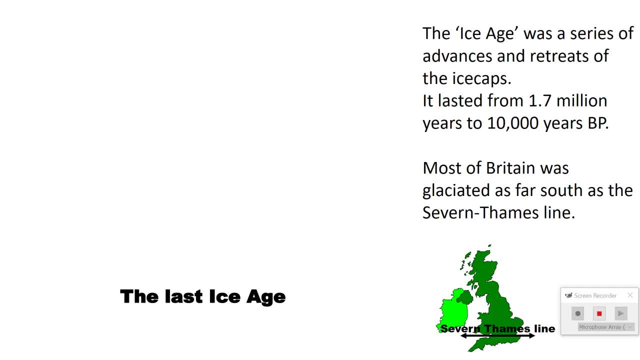 So just a bit of information for you: The last Ice Age. So the last Ice Age- was a series of advances and retreats of ice caps- And we're talking huge ice sheets, not individual places that stretched right down over Europe. And there's a line often talked about called the Seven Times. 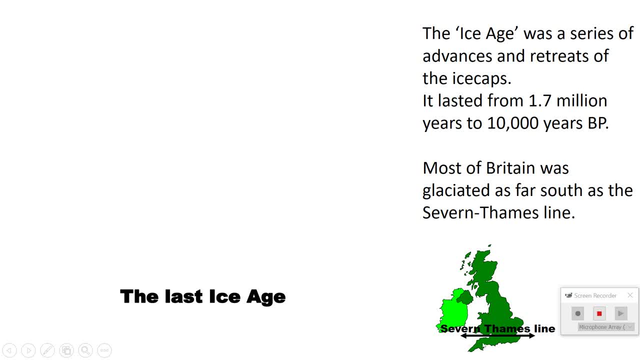 and Thames Line down by the River Thames, the River Severn And that kind of extensive where glaciation is meant to have reached in, and the UK- So that was they say about 10,000 years ago- was the last sort of point of where glaciation was still. 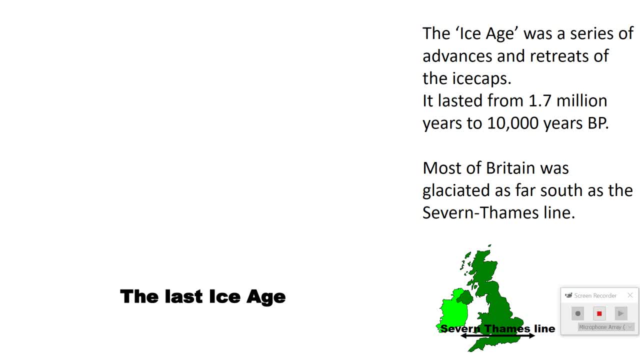 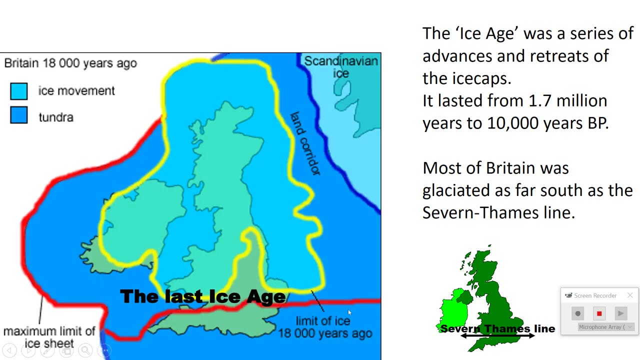 to this extent in the UK still going on. But the last glacial maximum, the furthest it reached down to Europe, was 21,000 or up to 21,000 to 27,000 years ago scientists talk about. So that gives you another date there. limit of the ice: This date is debated. 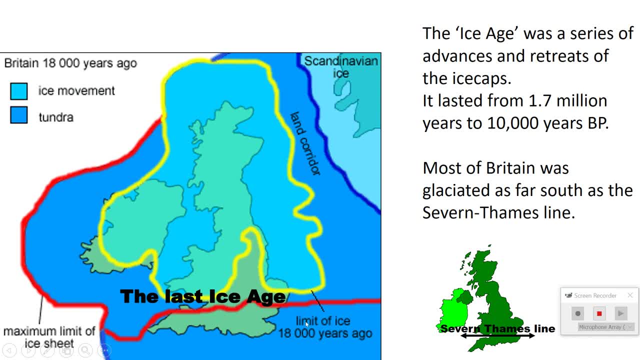 but between 18 and 26,000 years ago, that was the maximum And you can see huge amounts of ice and it would have been a nice sheet as opposed to an individual glacier. It was this series of advances and retreats, and our climate changes all the time. 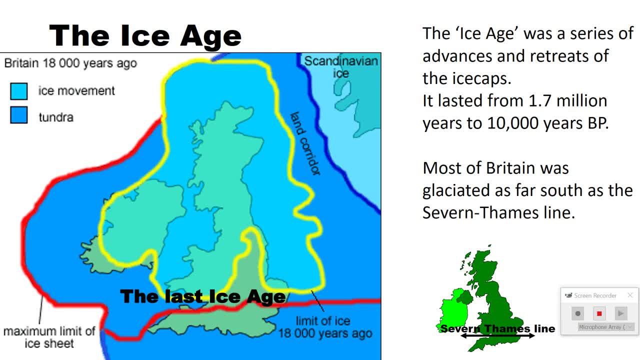 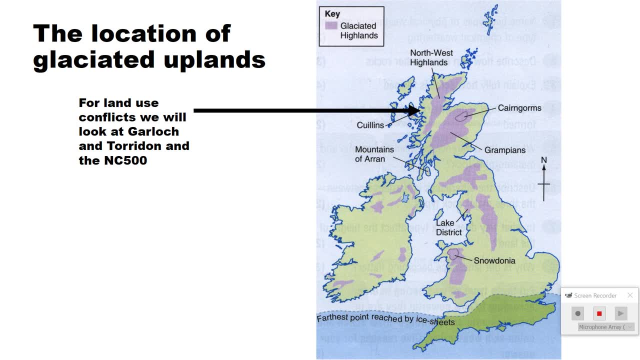 And we go through these glacial periods, what we call interglacial- which are a bit warmer. So we'll have a look at that in a moment too. The location of glaciated uplands in Scotland is particularly important. Scotland is effectively our case study We're going to be looking at. 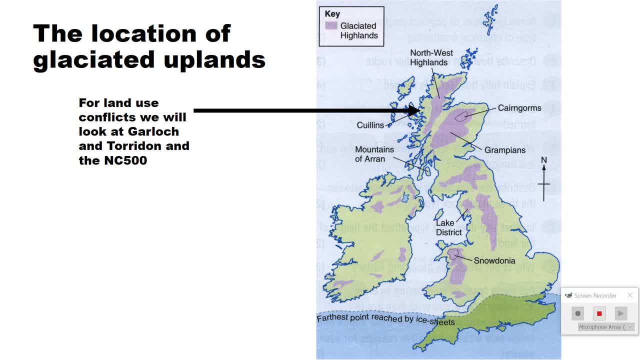 Gairloch, which I spelled wrong there, and Torridon, around the north coast 500, which some of you might have heard of. It's a route which comes across from Inverness and it tours this area about roughly 500 kilometers, I think, around the north west coast of Scotland And Gairloch and Torridon. 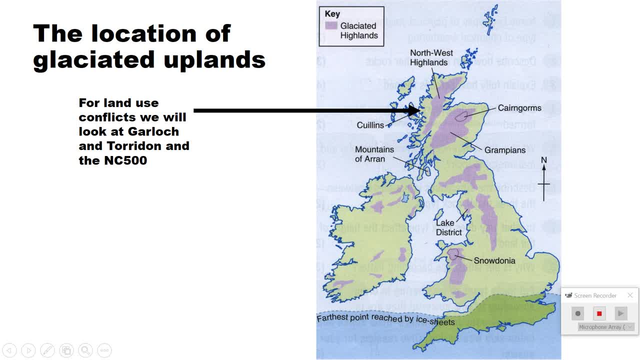 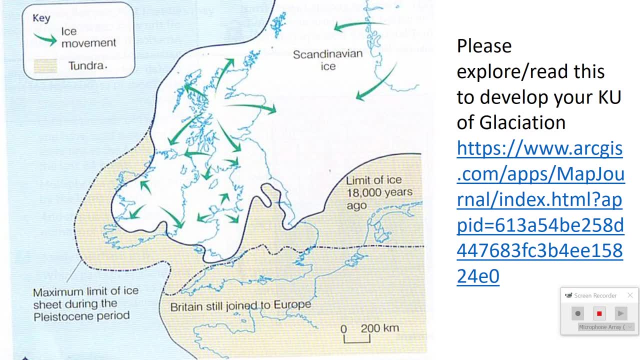 are located in around this area, kind of north of the island of Skye, north east of the island of Skye, And we look at land use conflicts there, as part of which is now a human topic. All right, there's another diagram showing you the Scandinavian ice sheet and limits of ice. 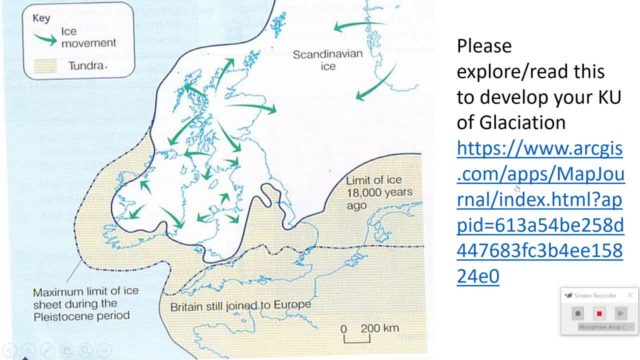 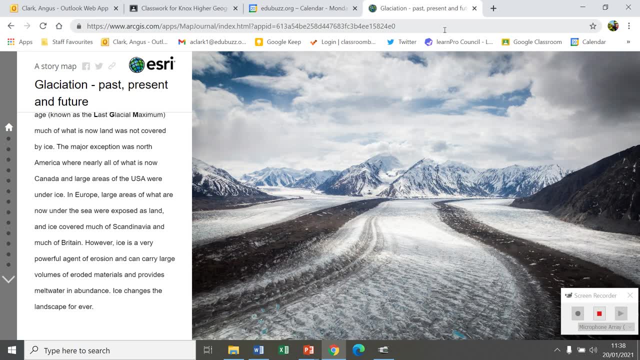 Have a little explore of this website here. I'll bring it up on the screen just now just to show you a couple of features, And it'll give you a bit of information about glaciation generally, in the past, present and future. Let you see some amazing photos as well. 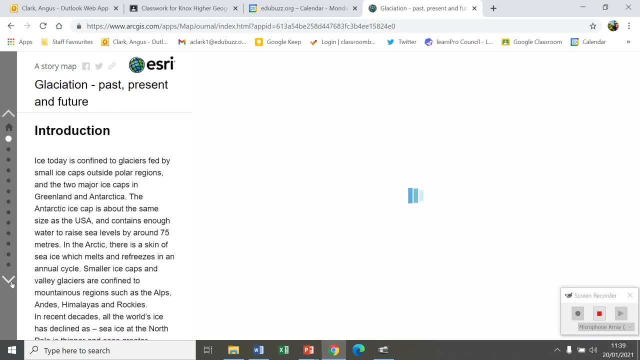 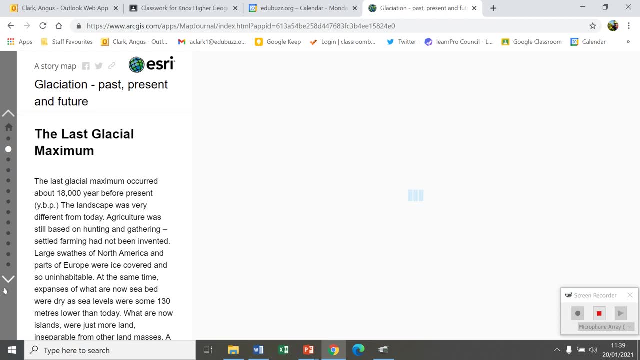 And this is what's called an ArcGIS story map. There's a lot of information on this And you can explore these maps that I've put up on the screen. They show and talk to you about the last glacial maximum 18,000 years ago, And it shows you these different layers within there. 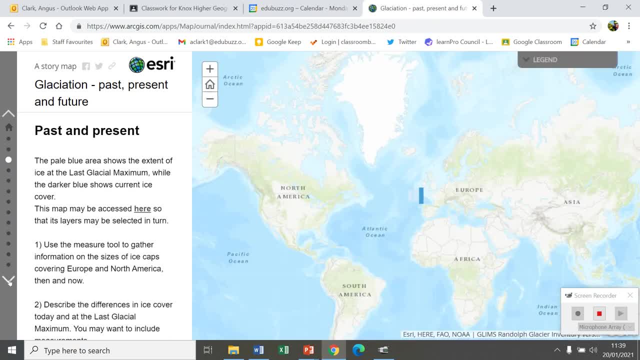 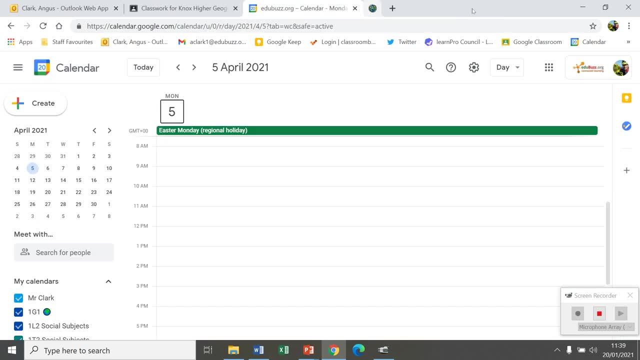 as well to have a look at. So there's a huge amount of information to go and have a look at, Have an explore, have a read, just to extend your knowledge a little bit. So I'll carry on with the presentation and you can do that yourself. This, as I was mentioning climate's. 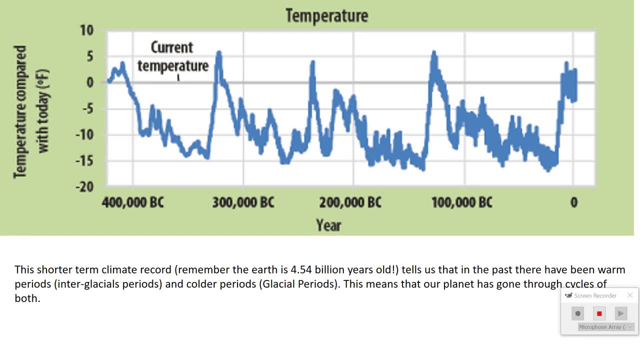 changing all the time over the course of our planet's history, from 4.54 billion years ago when the planet was created- That's how old we are- And we have these warmer periods where we see the temperature spiking above zero degrees Celsius. 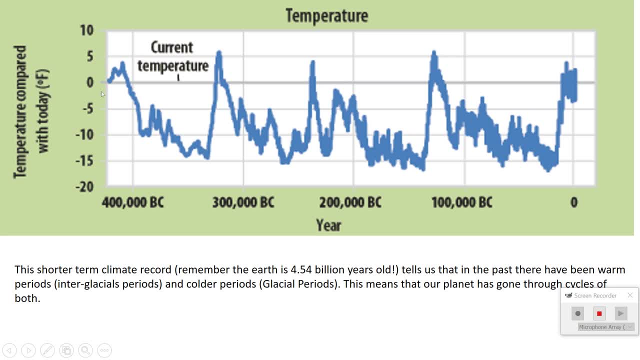 And this is compared temperature, compared with today. So today's average temperature is around 14 degrees Celsius on our planet And we know that's changing with climate change. We're getting warmer, But in the past our average temperatures have been much lower And you can see that these. 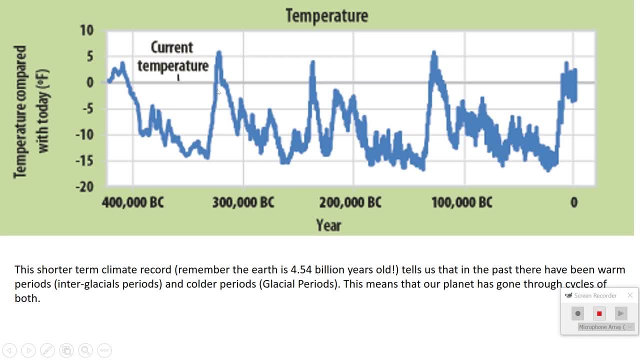 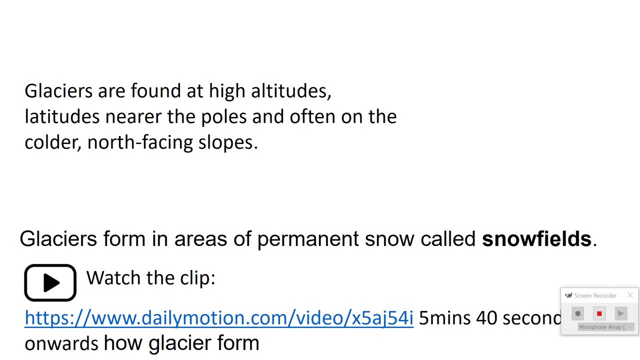 dips are periods of glaciation, and you could color these spikes as red and they would be our interglacial periods, where it's a lot warmer. So where do we get them? Effectively, glaciers form where there's permanent snow fields or permanent areas of snow, and they find at higher altitudes, In other words, higher mountains. 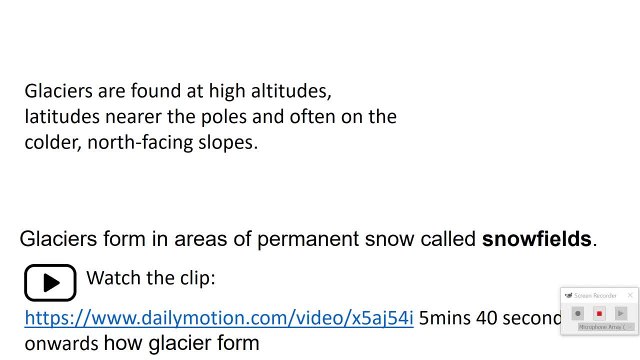 in other words and latitudes near the poles where it's colder. The effect of latitude in national geography on climate. it makes it colder further to the north And we've explored that. reasons to do with how the sun comes through the Earth's atmosphere and the curvature of the Earth. 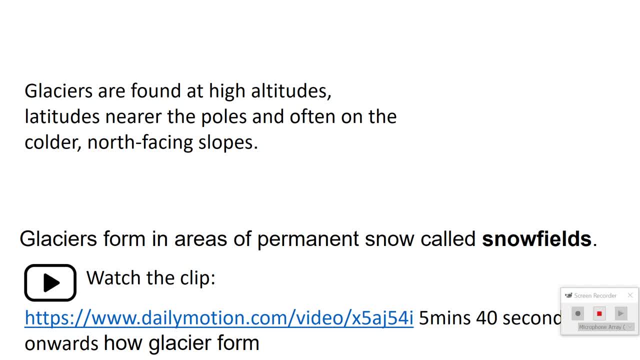 And we've also explored the north facing slopes And that's due to the aspect where the sun doesn't shine into the north facing slope as much, as much colder. So I'd like you to watch this video here from about five minutes 40 seconds, just for kind of a few minutes, And it really shows you quite. 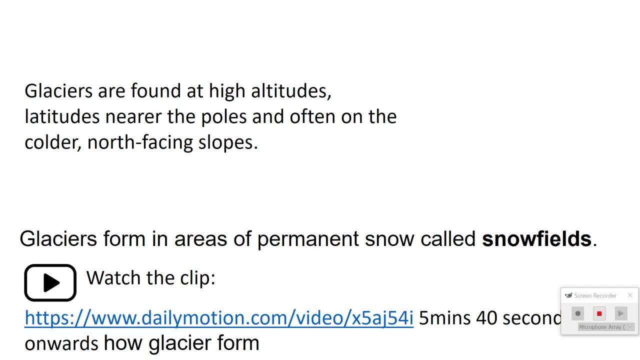 well how the glaciers form And we might watch a bit more of that in class at another point once we get back into school after lockdown. So you can see these. this is a glacier forming up here on the top right, much higher up. 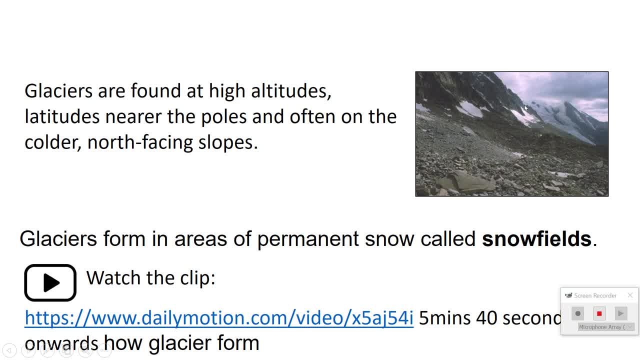 Above the general snow line in a north facing hollow, So it's actually what we call a Corrie- We'll come back to it later- And the snow is obviously going to fall because we've got more rainfall in the mountains as well, which falls as snow because the temperatures are colder. 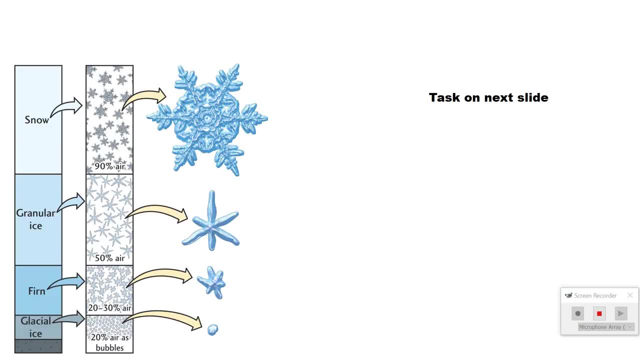 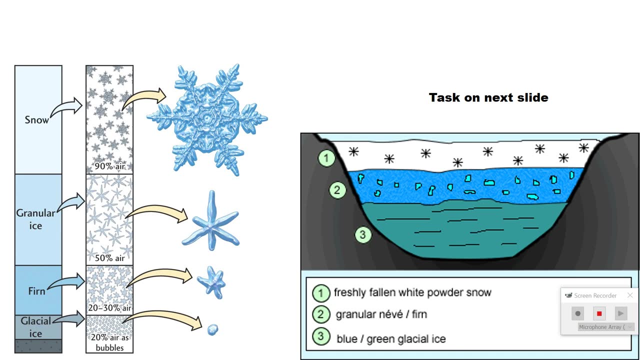 Okay, so what we're going to do? we're going to do a task on the next side, and it's just really about how glaciers form. So they do. they are created from snow which falls. We saw that in that last diagram of snow falling higher- but it compresses And 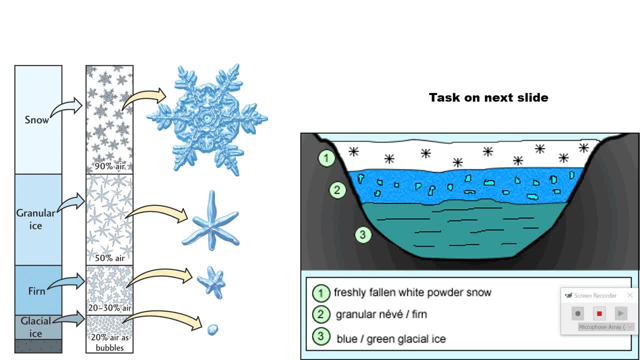 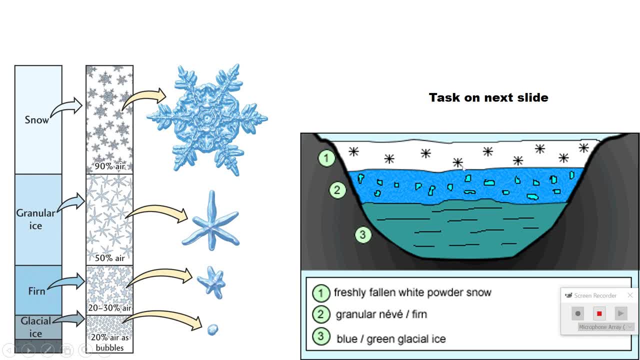 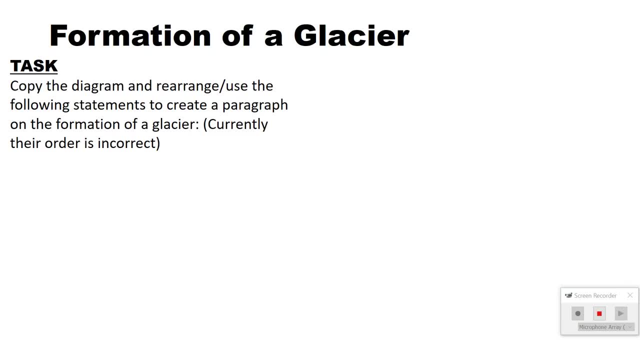 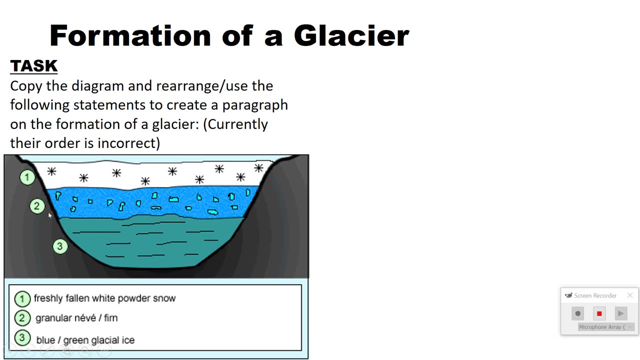 a powder to what we call neve or fern and then eventually into blue glacial ice. So what I'd like you to do is you're going to copy the diagram here into your notes. It doesn't have to be coloured particularly, but copy the diagram in with a key or just. 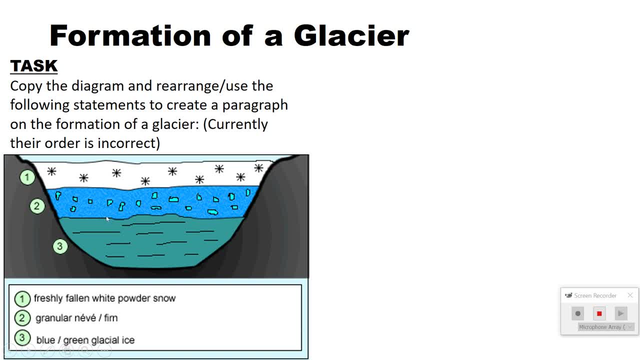 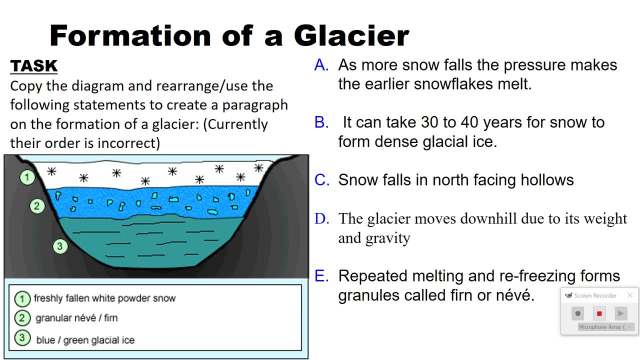 put these words in the spaces on your diagram And you're going to rearrange the order of these statements to help you explain the formation of a glacier. Okay, so that's your first task. The answer is on the next slide. you can pause this just now. 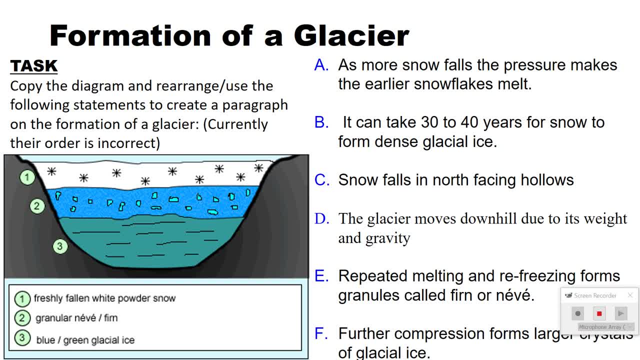 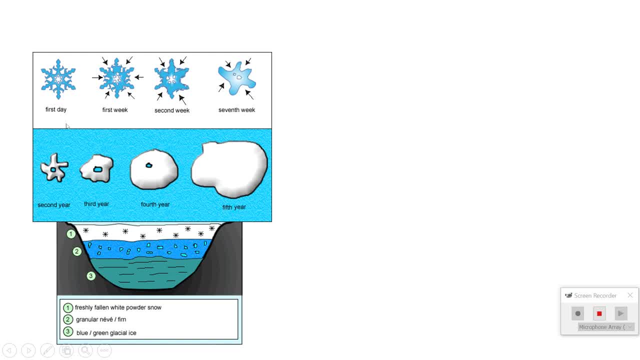 and then I'll go over the answer And you can make sure to check your work. So you've got that in your notes. Okay, what you can see is the actual ice crystals. they're all completely random, in actual fact. It's quite an interesting bit of science, And what we actually find is these ice. 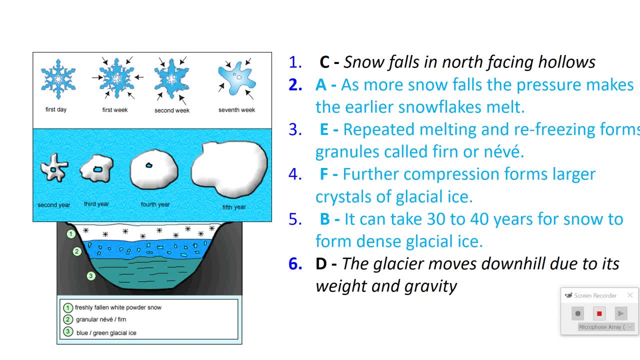 crystals. they compress and it melt a bit and they change form. So as they're compressed it changes and you see this first few weeks where the snow crystal changes, And after a few years it really changed form And we get this happening. So snow falls in the North-facing hollow. 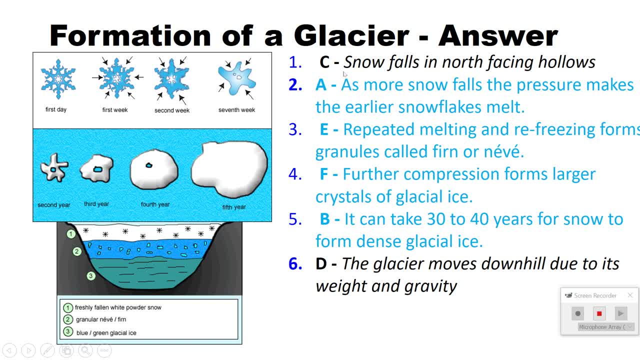 of what we generally end up being a corrie. and as more snow falls, the pressure makes the earlier snowfall lakes melt and repeated melting and refreezing reforms these granules into what we call neve. So this is this repeated freezing and melting. 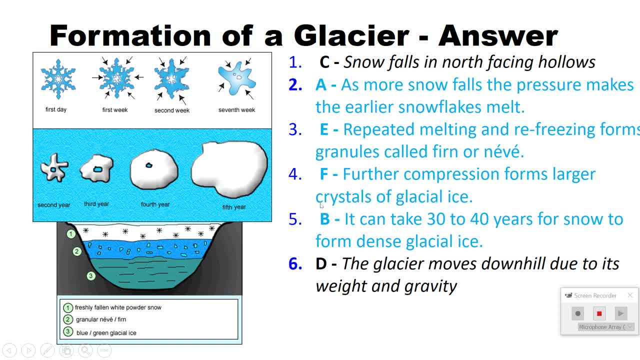 changing these crystals Further. compression forms larger crystals. They've got bigger glacial ice. It can take 30 to 40 years for snow to form dense blue glacial ice And then the glacier moves downhill due to its weight and gravity. So that whole paragraph that you've now got written out. 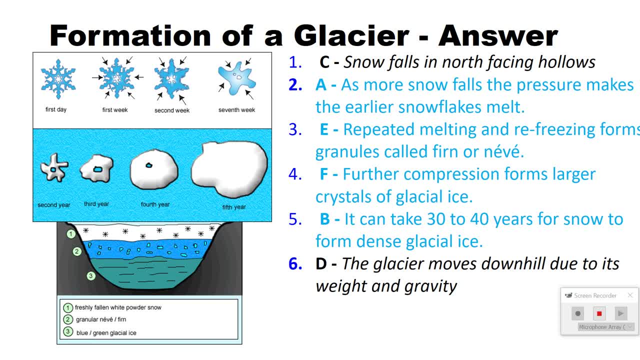 is probably a bit more than you need for the exam, Just to show you the kind of statement you'd need. snow is compressed to form fern, neve, then ice. It's one of the parts in terms of ice formation, But in actual fact you can get more marks than that. 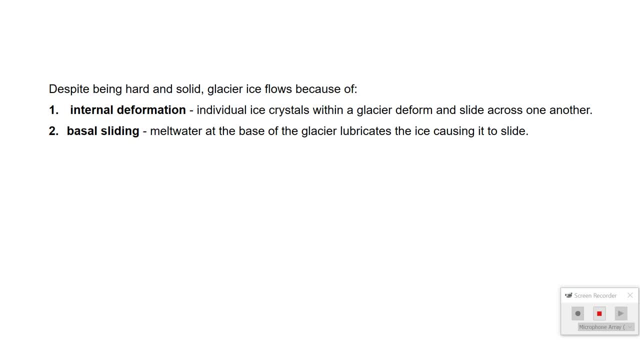 And I'll explain that later on when we look at features of erosion, about how you get your specific glacial formation marks in the question. So, despite being hard and solid, glacial ice flows because of two processes And if you mention these two, 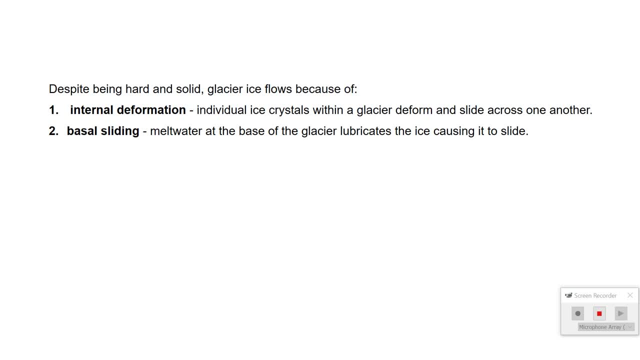 and I'll show you this in a minute. let me just write this down, these two processes. you get marks in the exam, So just it's probably worth noting down what internal deformation and basal sliding is generally from these descriptions. If you understand that, it's going to mean that when you recall information, 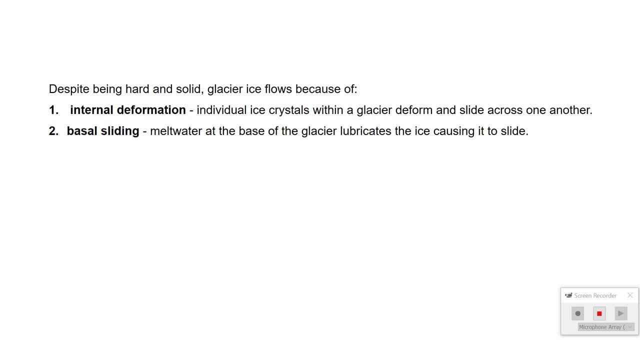 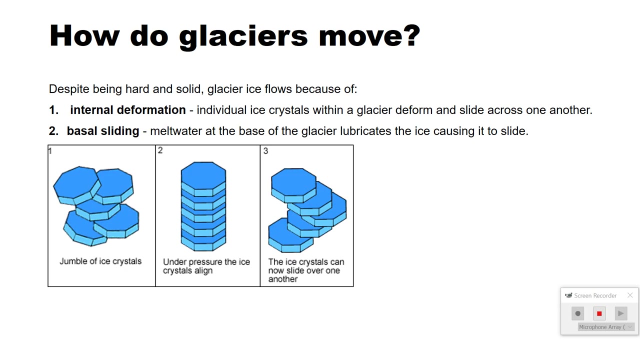 in a more simpler form. I'm just mentioning those phrases. you'll understand what you're talking about. So internal deformation is when the individual ice crystals in a glacier deform, they change shape and they slide across each other And basal sliding. so this is this. 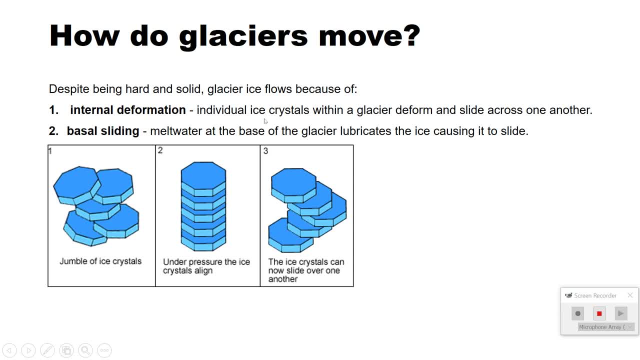 internal deformation and individual ice crystals in the glacier deform and slide. So under the pressure we've got these jumble of ice crystals and under pressure the ice crystals realign. they can slide over one another and that's internal deformation. 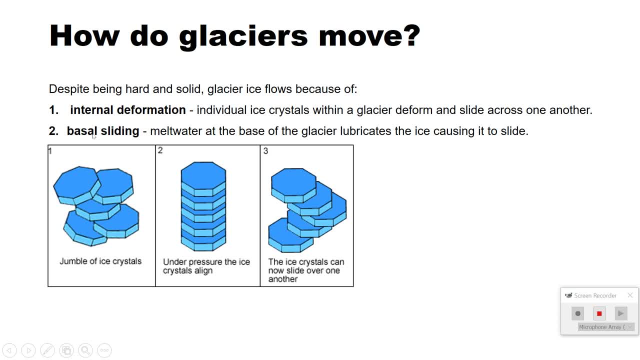 Basal sliding is just when we've got lots of water. So the glaciers are melting all the time at different parts or zones of the glacier, particularly in the zone of ablation, which is the melting bit in the bottom half of the glacier. 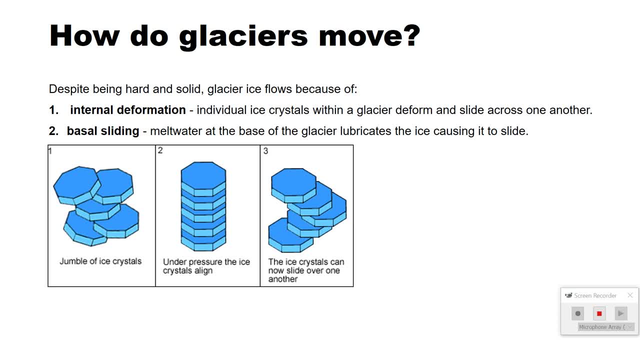 because it's lower down, it's warmer And because of all this water around the glacier, the water around the ice, it helps act like a lubricant, and like an oil on your bike chain, if you like, and it allows that glacier to slip and slide a little bit. 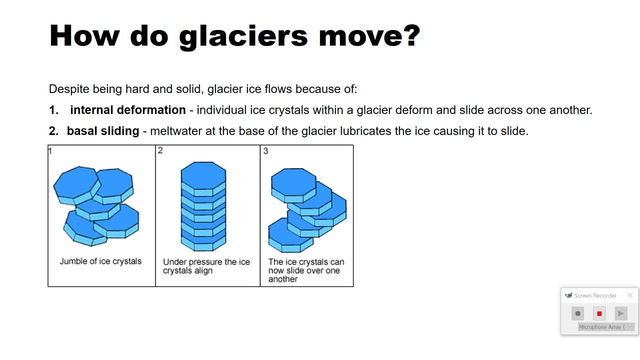 So together, internal deformation and basal sliding help the glacier move downhill due to under its own weight, due to gravity. So here we go. How do you get this information for gaining a mark in the exam for glacial features? And really I wouldn't get you to copy the diagram down. 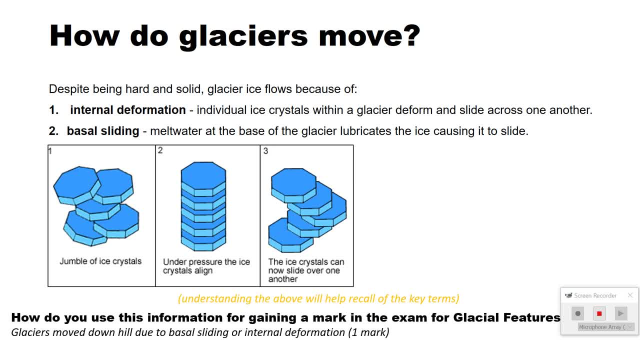 That's just to help with your understanding there. I'll just get you to think about this idea that glaciers move downhill due to basal sliding or internal deformation, And that would simply be enough to get you a mark in the exam about their movement. 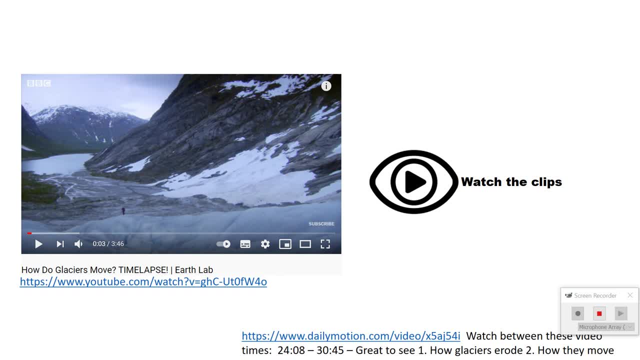 Right Watch the little clip here. I'm not going to play it within this presentation. You can do that on the presentation. you've been given The link's there too, And there's a little time lapse with the glacier there as well. 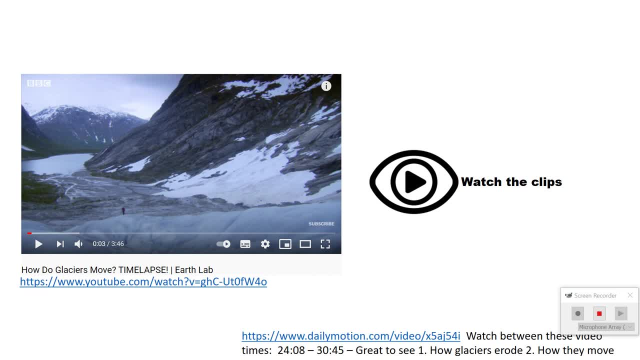 It gives you an idea about how they're working there. And, more importantly perhaps, is another clip from the blue, the Ian Stewart documentary about the power of the planet ice. So if you watch the clip there between 24 minutes and 30 minutes, 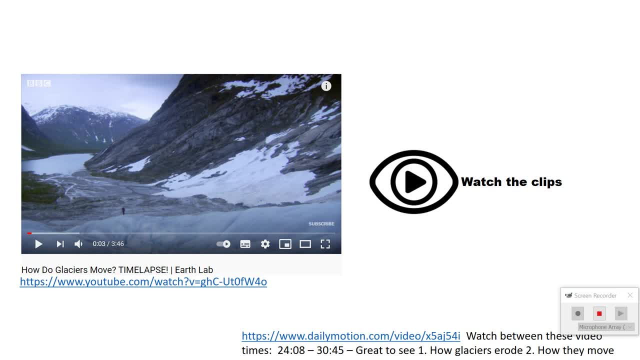 you get a really good idea to see how glaciers are rowed. It's really interesting. They get to kind of go in and see all these different features of the glacier and it sees how they move as well. So go and watch that as well for your learning. 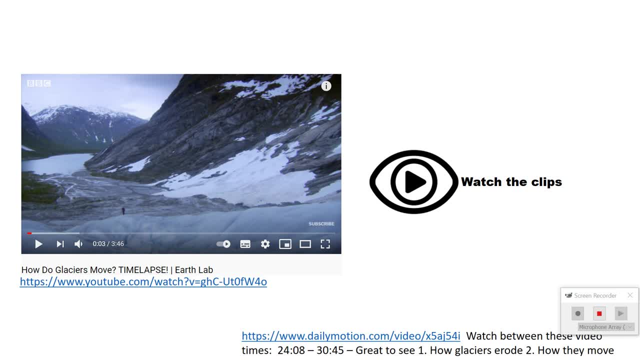 And that'll really kind of bring some of that to life for you. They're really amazing things to go and see. I remember years ago going to Commé Aire in France- Italian border- and looking at the Val Forêt glacier And we did some studies on it. 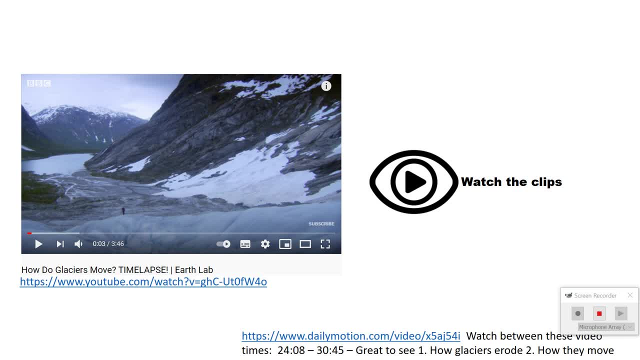 And it is amazing. It's amazing to get out and do field work on these things, walk about on them and have a better understanding about how they work, how they change and shape our planet. So they're quite interesting features. So I'll tell you a bit about how they move. 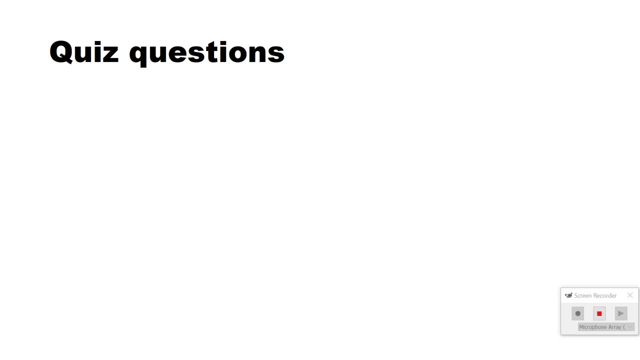 Some quiz questions. See how you get on with these. You can pause the slide at any time and write down your answers, And maybe you could submit that with your other work. You're going to send pictures in of it to me, or you can do it in a Google Doc and send it in to me as part of this assignment. 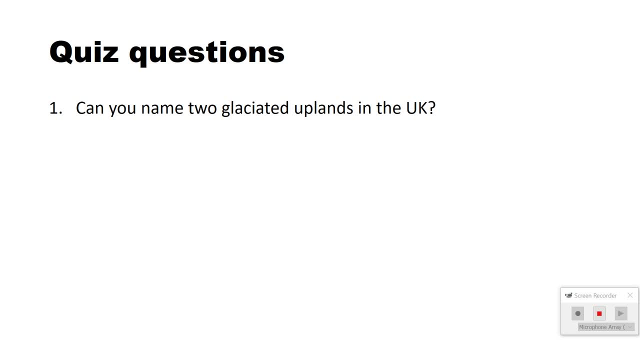 So can you name two glaciated upland areas in the UK? You might have to go back and look at the slides there. There is a map on one of the pictures you can have a look at. Where would you find glaciers? Okay, 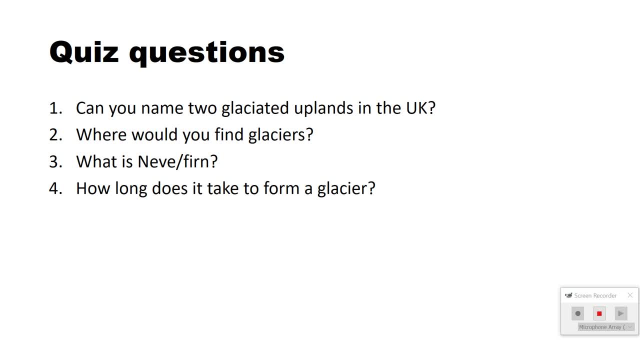 What is Fern Neve? How long does it take to form a glacier? Glacier flows move in two ways. Can you name them? So I'll just kind of go over those Glaciated air and upland areas in the UK. You've got the Cairngorm area and you've got the Northwest Highlands. 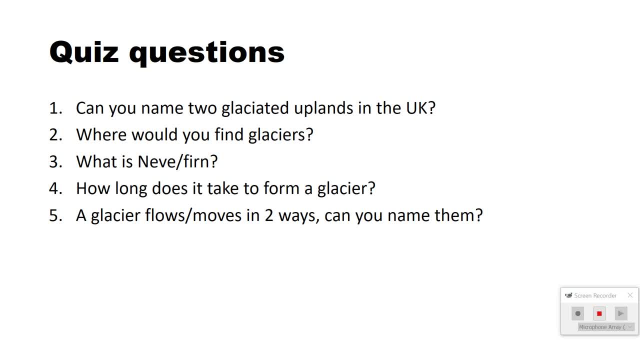 You could talk about either of those which is known as the Grampian Mountains. Where would you find glaciers? You should have got the idea You're going to find them high up in mountain areas and also at higher latitudes. So we're at 57 or 55 to 56 degrees north down in Haddington. 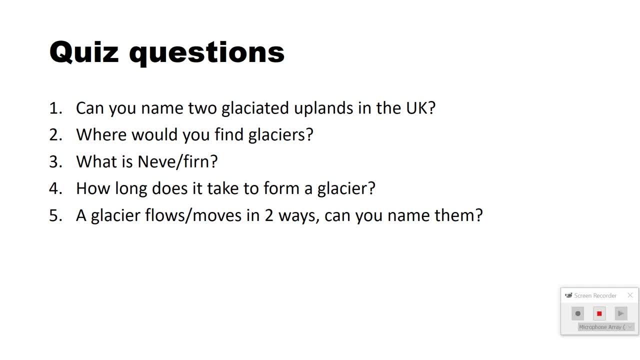 But really you're going to find them generally at higher latitudes than that, Or at higher altitudes where you might go to Alps, the Alps where you're talking 3000 meters and above and that kind of height And for some of the top of the mountains. 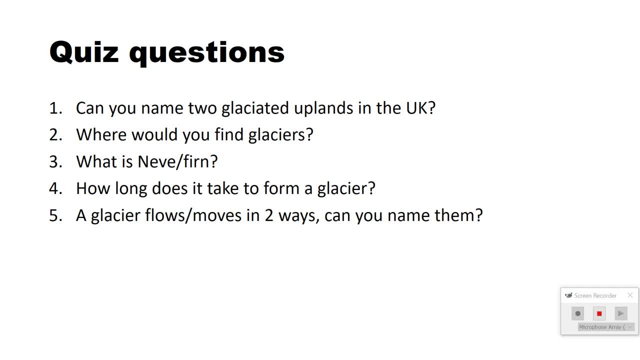 What is Fern Neve? Fern Neve is the snow that's been compressed. It's not quite got to be in glacial ice yet. How long does it take to a glacier to form? I think from rightly on that slide it's up to kind of 30-40 years. but these numbers 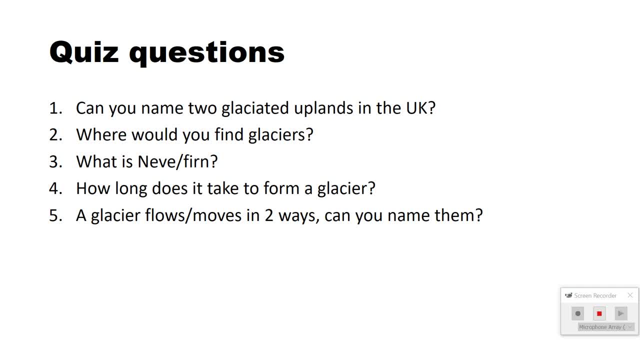 you'll find different quotes for them. It's not something that's key for the exam. A glacier flows moves in two ways. Can you name them? Hopefully you've remembered internal deformation, Which is the ice crystals aligning So they slide more better on top of each other. 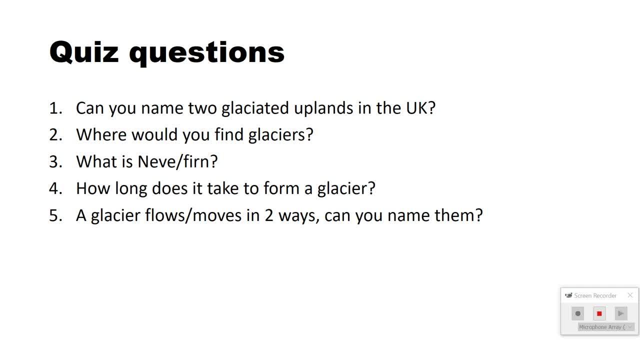 And basal sliding, which is when all the water and the melting water on the actual glacial ice lubricates the glacier and allows it to flow downhill due to its own weight and gravity. Okay, So if you watch the little clip here, there's a little additional bit of information. 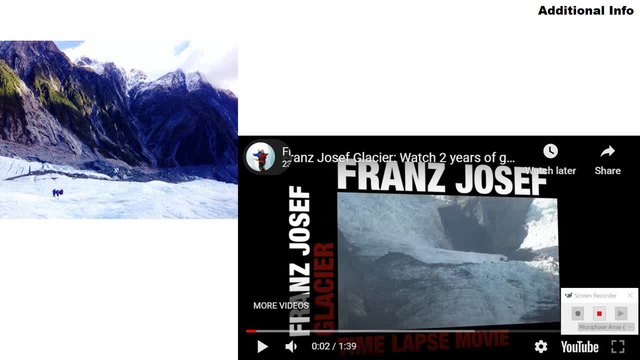 about the Fran-Joseph Glacier from France And it kind of shows you the changes that are happening because of climate change around the world And a lot of our glaciers are disappeared And for places like the Himalayas and the countries below them, there's going to be. 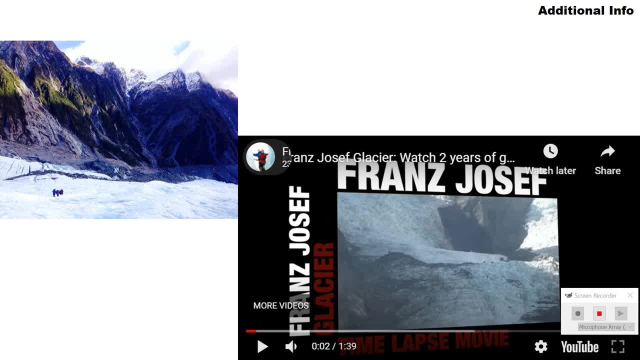 huge water scarcity in the future. The dry season happens or the dry monsoons taking place, where people rely on these waters from melting glaciers during the summer months to have enough water to farm crops. They're not going to have that if glaciers completely disappear. 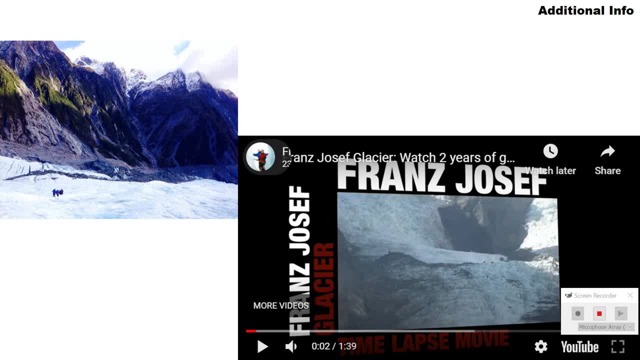 And there's going to be huge, probably, amount of migration and forced migration because of climate change really. So there's kind of links into another topic there, Moving on some other sort of photos to show you that as these glaciers roll, they're going. 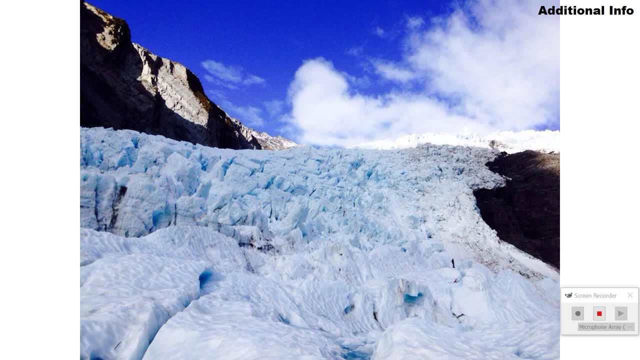 to act like almost like a river of ice and rolling around the scenery And they can have huge crevasses, cracks in the ice that people can fall into, And there's a man just standing here to show you the scale of how big these things are. 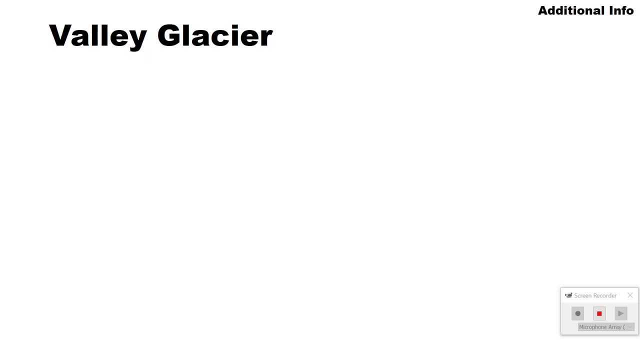 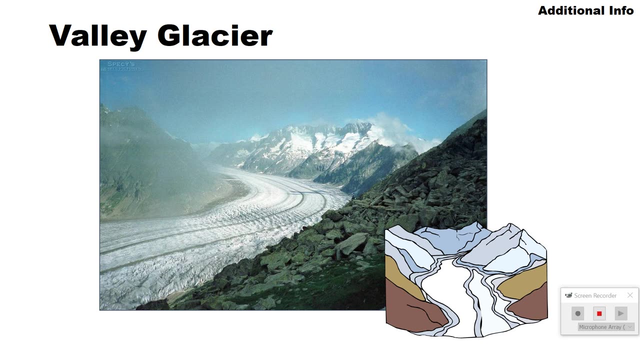 And just some more pictures. Okay, a valley, glacier, Valley. glaciers fill a valley funnily enough, So you can see one here. This is a huge example, And you can see all these great lines And these are what we call sediment in the glacier. 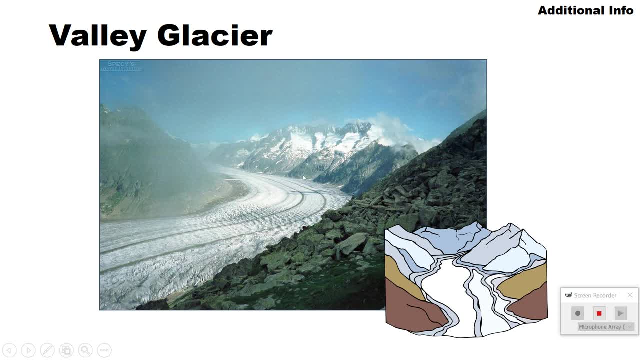 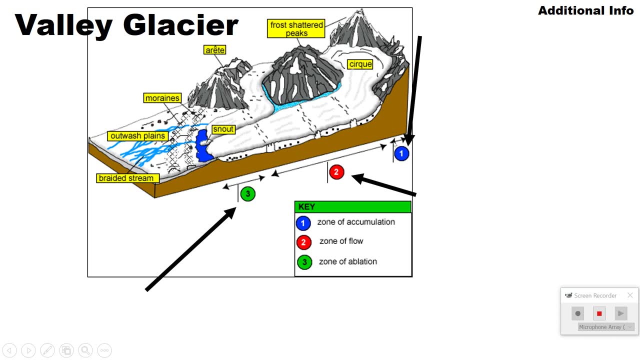 We'll come on to what these are called later in a future lesson, Some sort of key features of a glacier. We've got zone one So you can see on this area here And there's something called a cirque in the Alps. 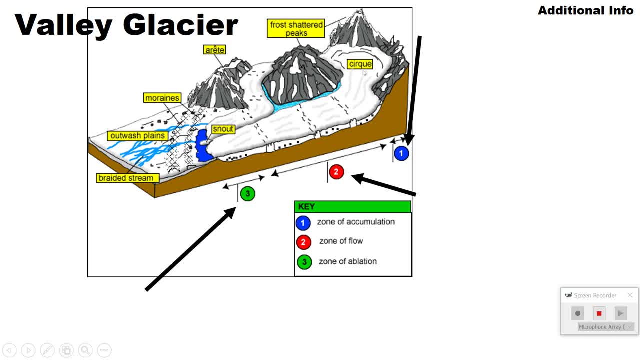 They're called cirques, in the UK They're called corries, So they're kind of a hollow shaped depression and which get kind of carved out into a bowl shape And that's where the glacier generally starts And we get frost shattering. 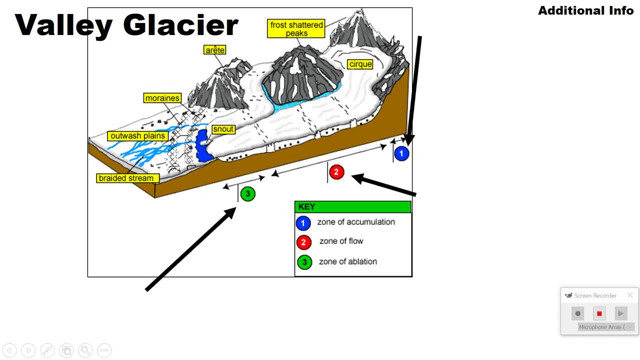 That's that free fall weathering on the peaks that can add these sediment to the glacier And you saw that in the picture, These great bits of rock on the glacier. We've got the zone of flow which is this kind of central area to the glaciers, kind of moving. 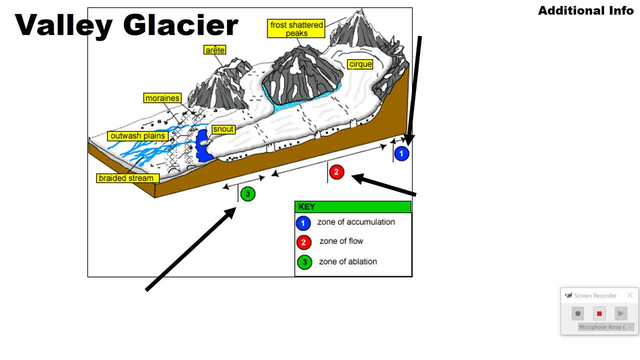 And because of that internal deformation or basal sliding, And at the front we've got what's called the snout of the glacier. That's the front of it, Okay, And what's sometimes called the terminus, And then we've got different Marines. 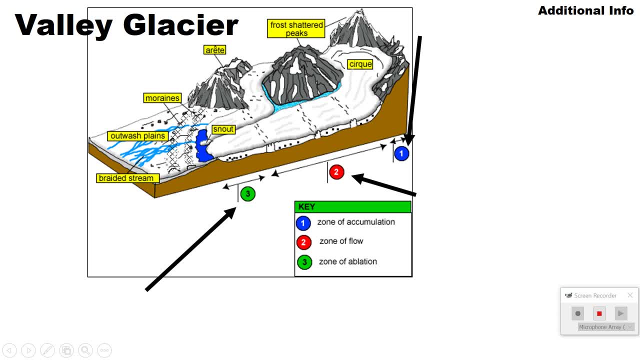 We'll look at Marines at a later date. These are where sediments are dropped off and the glaciers obviously melted back a bit, having been up here at one point, And there's some other features there too. There's also what we call an equilibrium line. 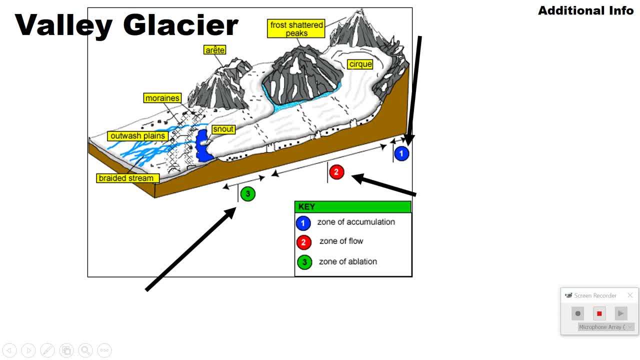 And that would be kind of around halfway here You can see on the monitor, And that means that's the place where there's not more melting or accumulation of snow, And it's a perfect balance. That's why it's an equilibrium line. 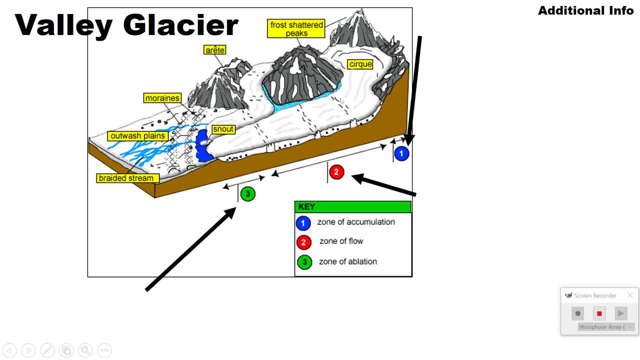 Anything above is generally known as the zone of accumulation Number one, where we've got a build-up of snow, and zone three is zone of ablation. Well, generally we've got more melting of the glacier than we have build-up of snow. 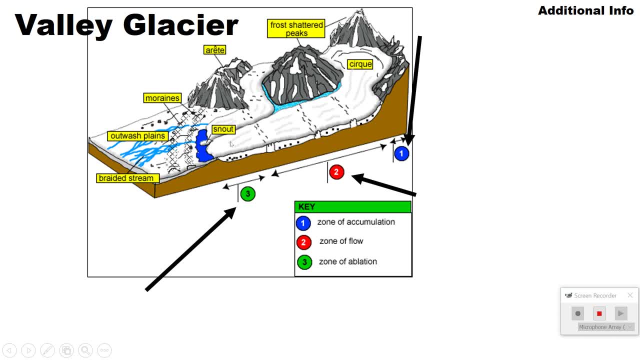 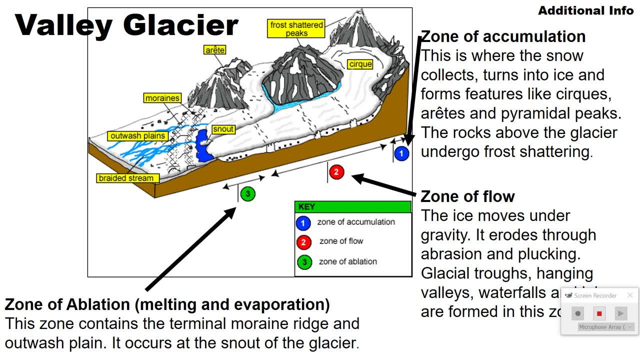 So the equilibrium is in the middle. So there's some little points about that there. I'll let you read those yourselves and you don't specifically need to know this for the exam. But it is quite useful to understand what zone of accumulation and zone of ablation and what the 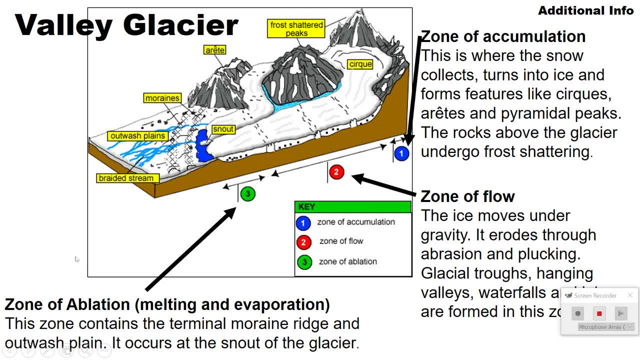 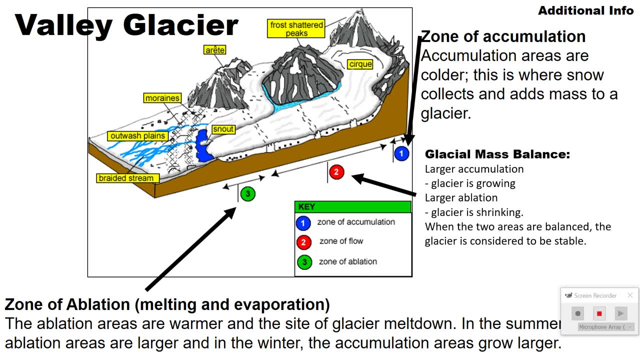 glacial snout are. So if you take a note of what the zone of ablation and zone of accumulation and the snout are- just for your own knowledge for this topic, it will help you understand. So that's the sort of key bits you can note down there. 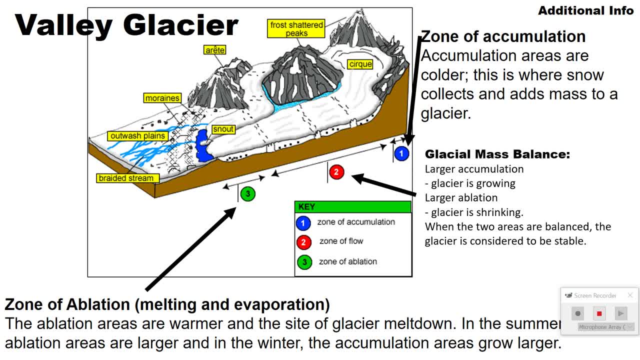 So glacial mass balance? All that is is a larger accumulation- The glacier grows- and a larger ablation- The glacier shrinks- And that's what we call about a mass balance. When two areas are balanced, the glacier is considered to be stable. 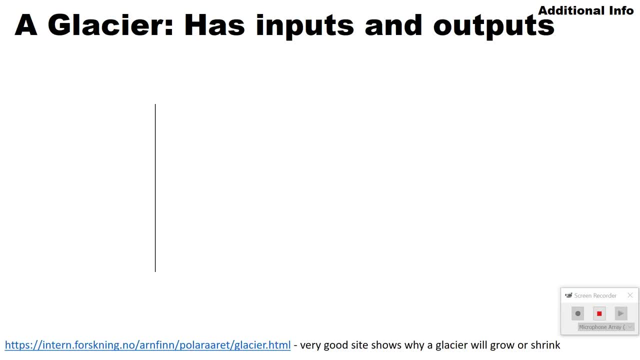 And that's just additional information there. So a glacier has inputs and outputs. Okay, there's the glacier coming in Zone of accumulation, That's our inputs and that can be precipitation in the form of, generally, obviously, snow in the mountains, And we've got avalanches that can drop into our corey from above and a zone of ablation. 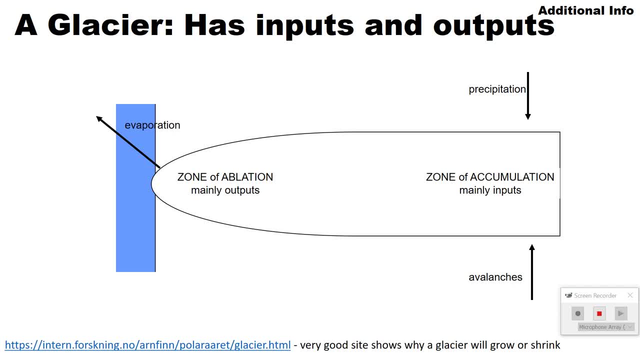 That's our outputs, and quite often that's a form of evaporation, because it's much warmer as well and melting and melt water streams coming off And sometimes, if it's by the sea, we can get something called glacial carving, which is, I guess, where the glacier gives birth to icebergs. 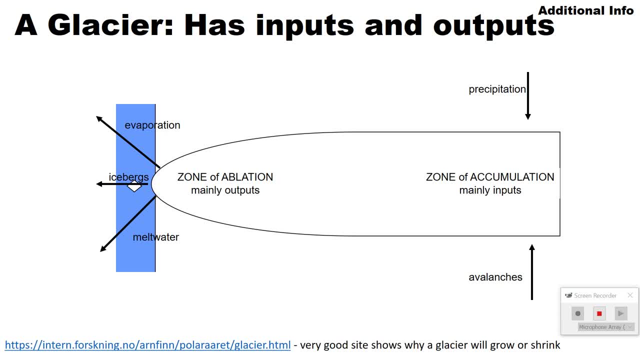 If you want to think about it as calves and cows and giving birth to icebergs, There's an app here which is have used in the past. It's really good. It won't work on the school computers, But if you can get that to, 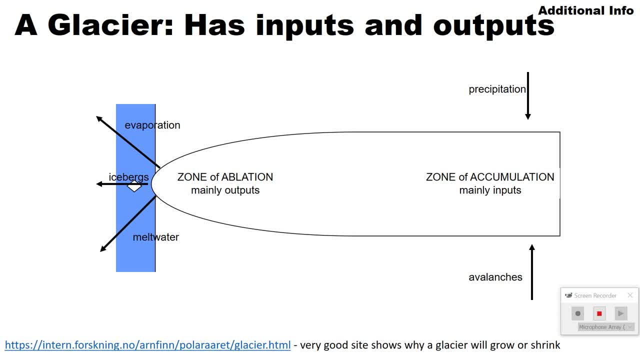 Work at home. Brilliant: It gives you a really good idea about how glaciers can ablate, or ablation or accumulate, and you can change the temperatures and see your glacier change in size and shape. So brilliant and little bit of software just to get a bit of understanding about how glaciers work.